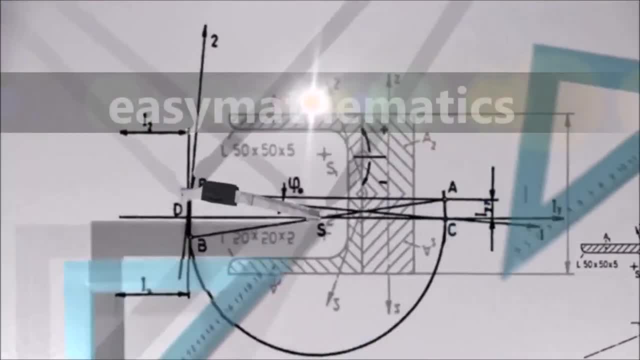 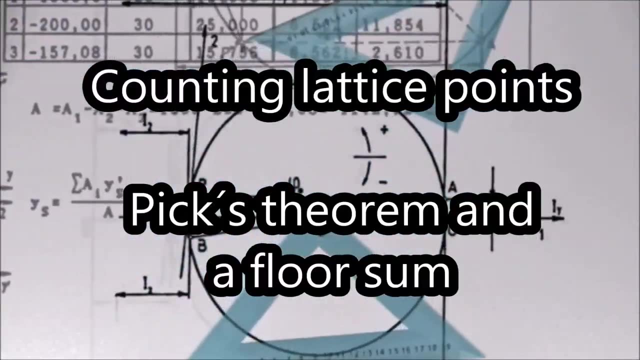 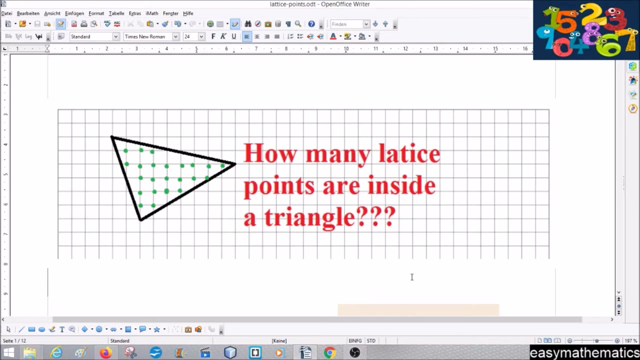 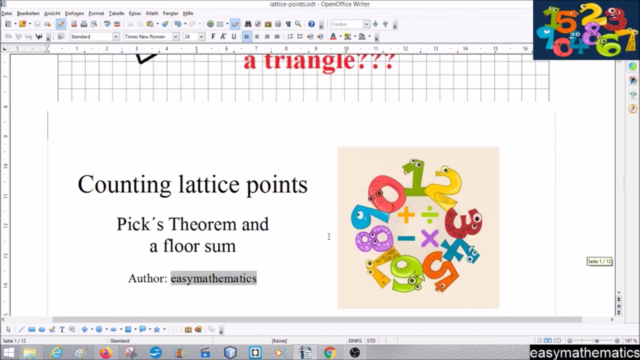 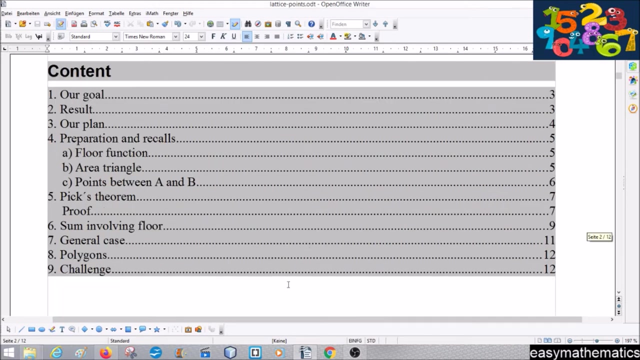 Welcome to IseMathematics and a new video. How many lattice points are inside a triangle? We count lattice points with Pick's theorem and we will also evaluate our floor sum related to these problems. All right, okay, so first we specify our goal. 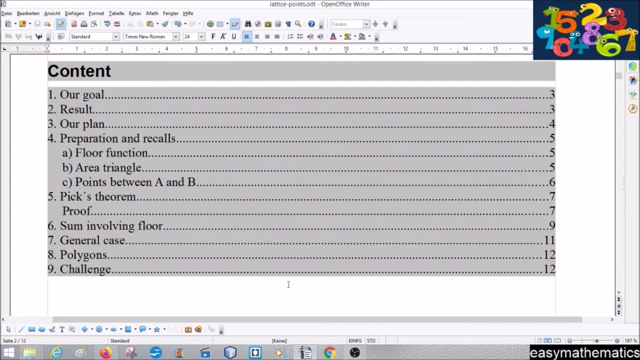 Then I show the results. Then I want to talk about the detailed plan. Here we prepare some definitions and we make some recalls. Then we talk about Pick's theorem. We will prove it for special cases. Then we will discuss the sum involving the flow function. Then we discuss the general case and before we 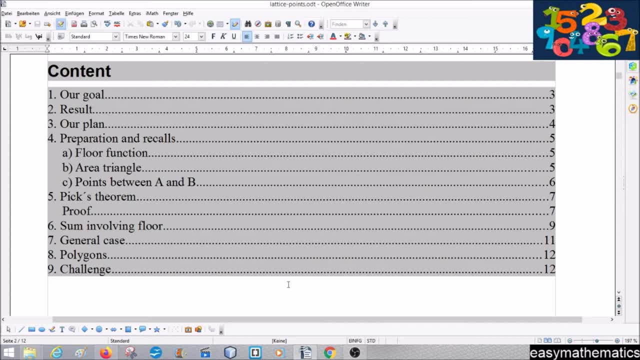 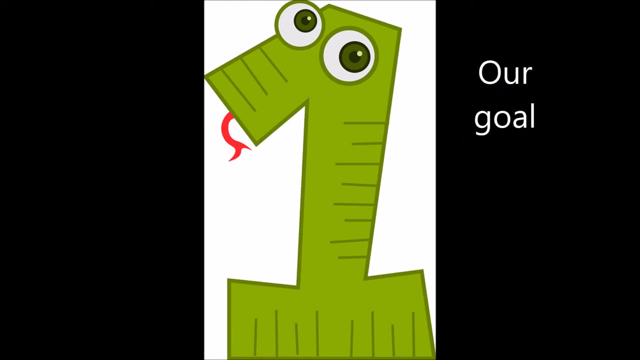 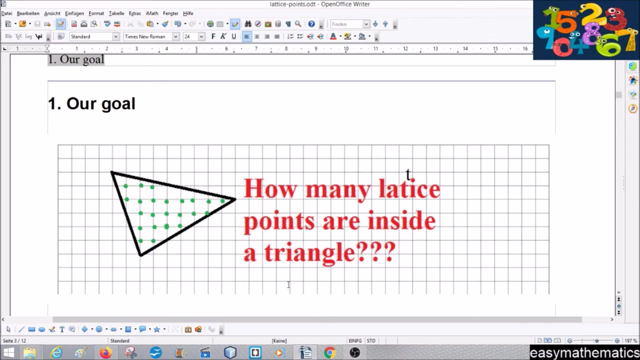 end. here we generalize the counting problem from triangles to polygons, and the last point is a challenge. So what is our goal? Our goal is, if we have a triangle with integer vertices, then we want to count the points inside the triangle with integer coordinates. difference between 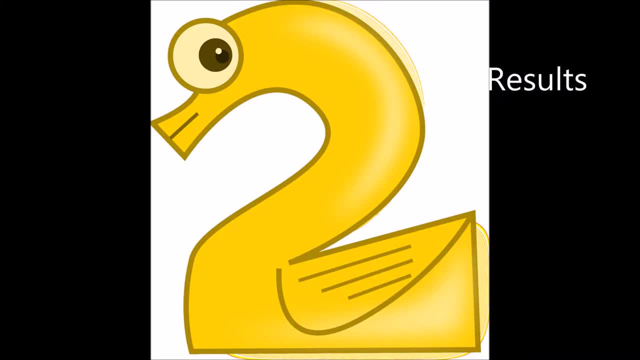 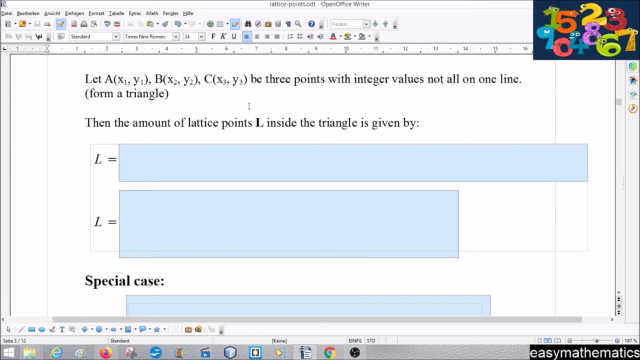 two points. Okay, Yeah, Yeah, see, with integer values not all on one line, so they form a triangle. in other words, then the amount of lattice points, capital L, inside the triangle is given by following expression: 1, half times the absolute value of, yeah, this difference. 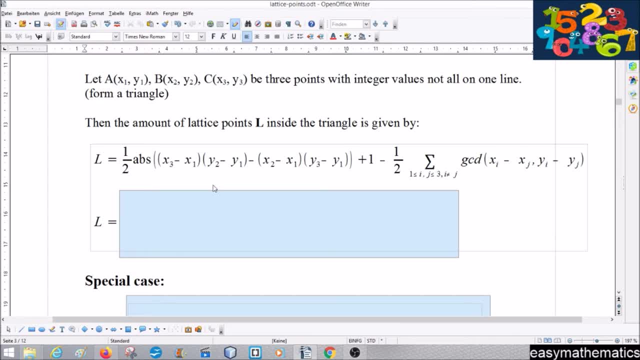 x3 minus x1 times y2 minus y1 minus x2 minus x1 times x3 minus y1, y3 minus y1 plus 1 minus 1 half. the following sum: i and j. they run from 1 to 3 inclusive. i. 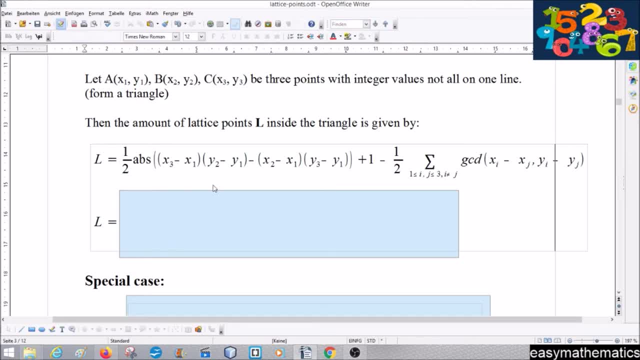 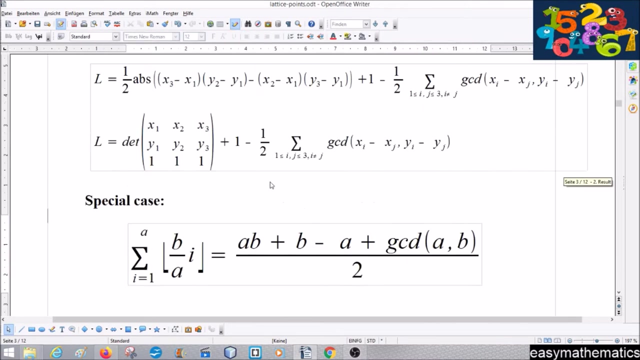 not equal j, and we sum up over the gcd of the coordinate differences. okay, and the first expression, the one half times the absolute value. we can write this also with a determinant. this is the area of the triangle, okay, and the special case is this sum. we will see how we get the special case, so 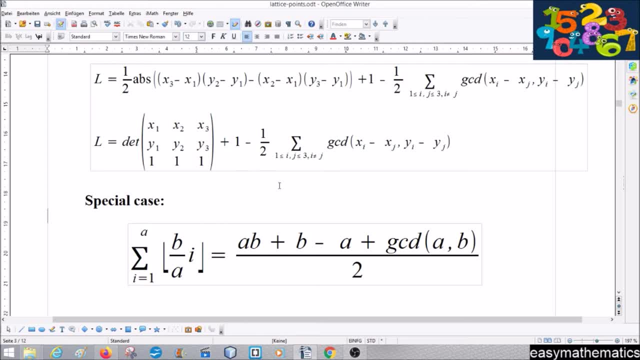 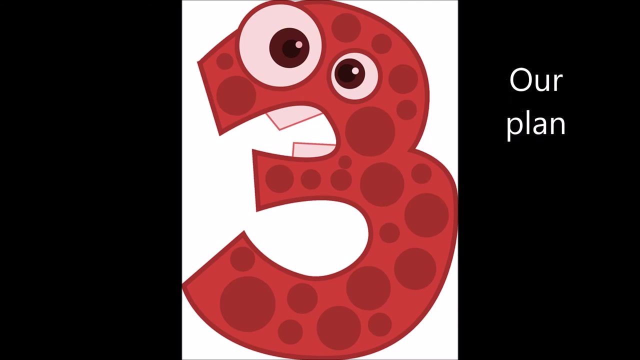 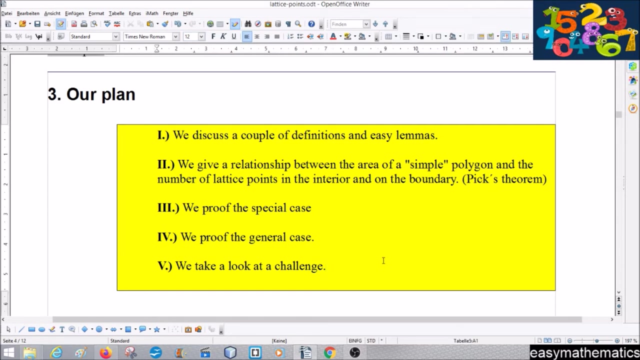 the sum from i equals 1 up to a over the floor of b over a times i equals a times b plus b minus a, plus the gcd of ab over 2. and i should mention here ab are positive integers, so our plan more detailed, okay, so first we discuss a couple of definitions and easy lemmas. 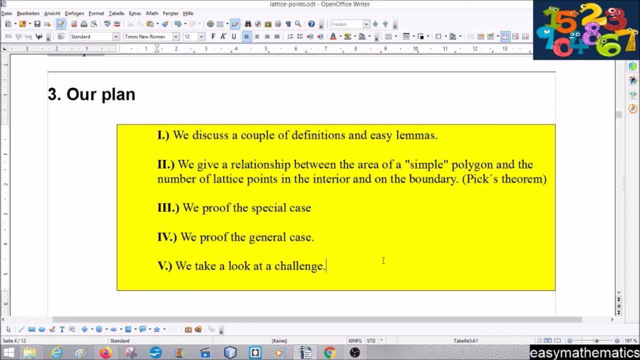 then, second, we give a relationship between the area of a simple polygon and the number of lattice points in the interior and on the boundary. this is called pig's theory. then we first prove the special case, then we prove the general case, yeah, and then we take a. 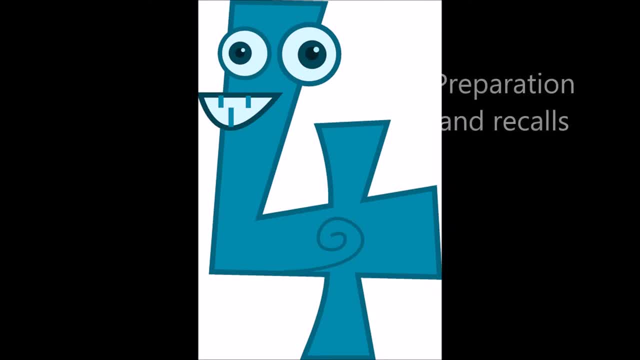 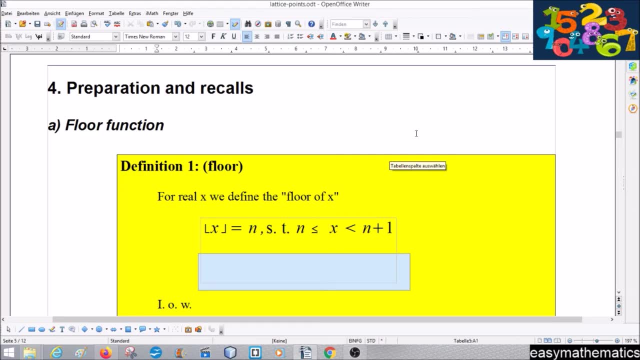 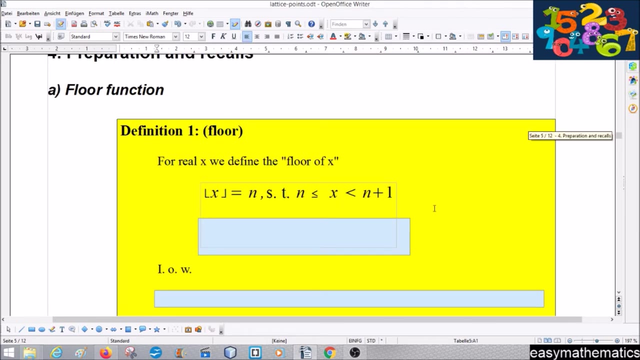 look at the challenge. so first, the floor function for real X. we define the floor of X. and the floor of X denoted with this: yeah, braces with the foods. yeah, it's. this is a natural number or it's an integer, and what kind of integer it's? 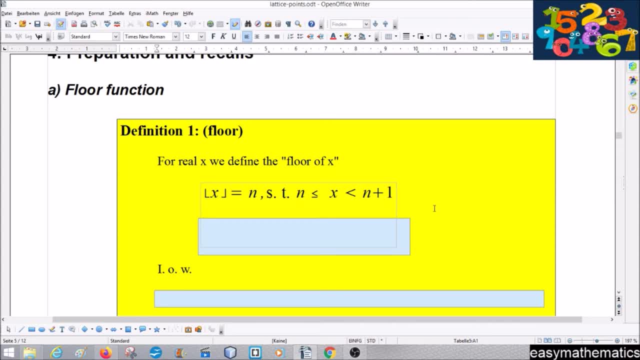 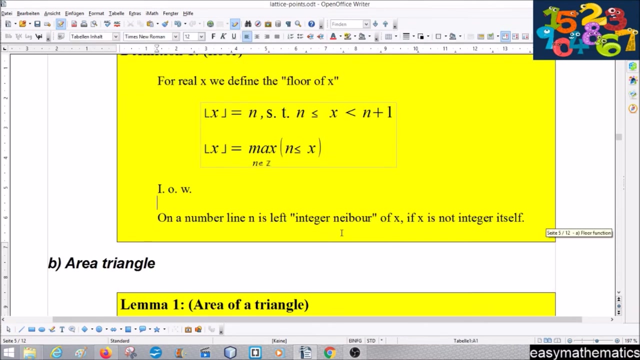 an integer in such a way that X lies inclusive n and exclusive n, plus one. another definition which you will might see is this: one floor of X is the maximum over all integers less or equal to X and, in other words, on a number line, n is the left integer neighbor, so the most left integer neighbor of X. all right, 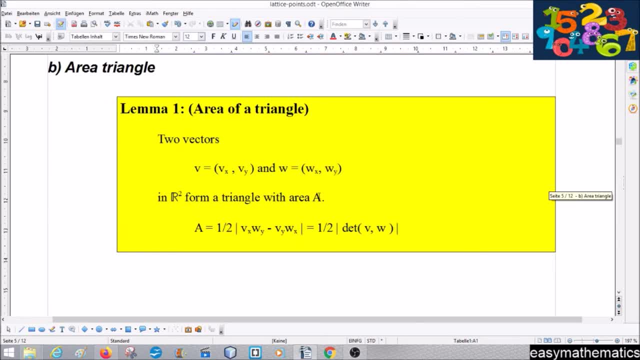 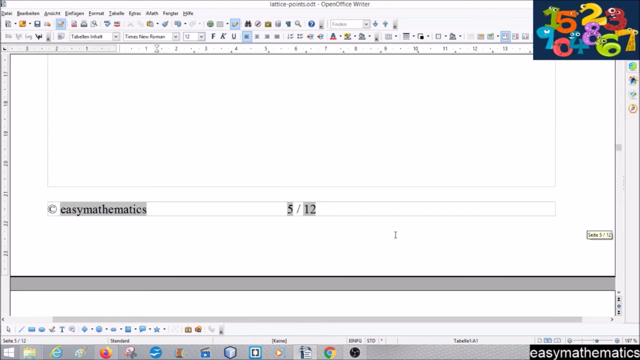 then be the area of a triangle. yeah, a. well, and when two vectors, B and W, they form a triangle, then the area is given by one half times the determinant, and if we are not sure about the mathematical orientation, we use the absolute values here. okay, and then the third one. 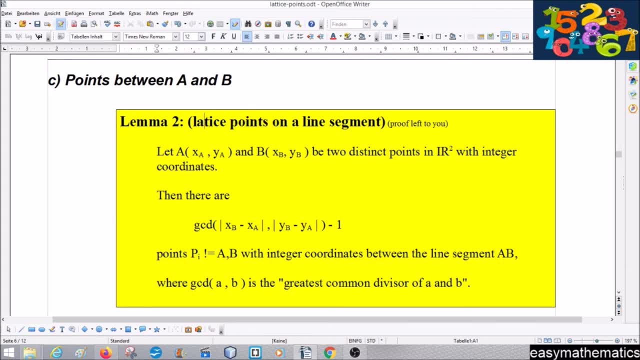 The second lemma is lattice points on a line segment. If we have a and b, two distinct points with integer coordinates, then they are gcd of the differences minus one points, pi, not a and b, with integer coordinates between the line segments. And gcd of a- b is the greatest common divisor of a and b. 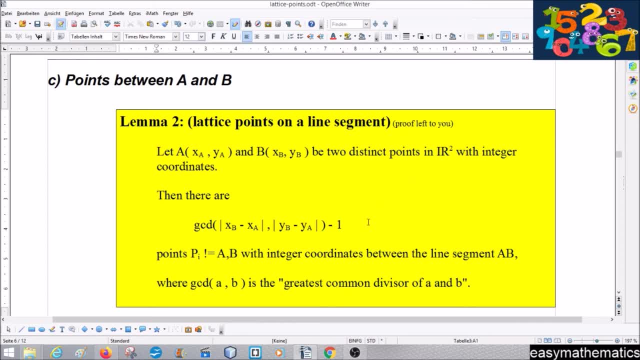 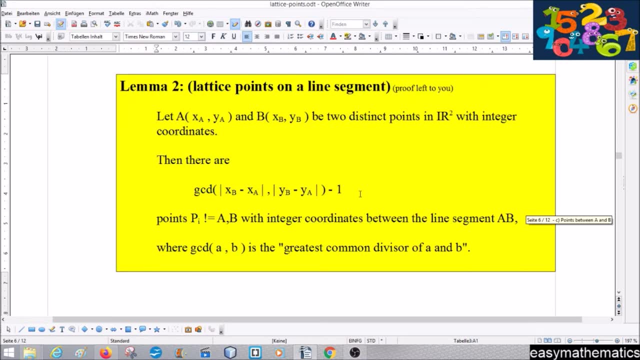 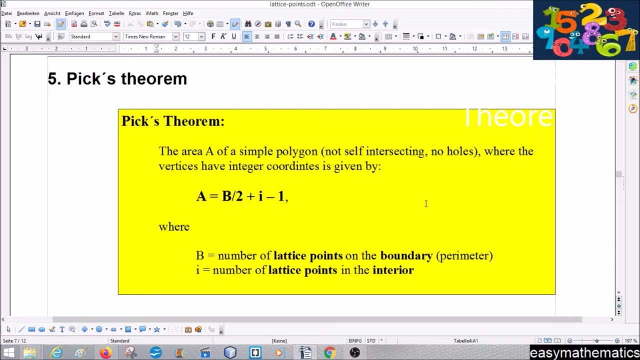 Alright, and the proof is left to you. We will continue, We will use this lemma, but I will not prove it. It's not so difficult to show. I'll leave that proof for you. Okay, The area a of a simple polygon is not self-intersecting, and no holes. 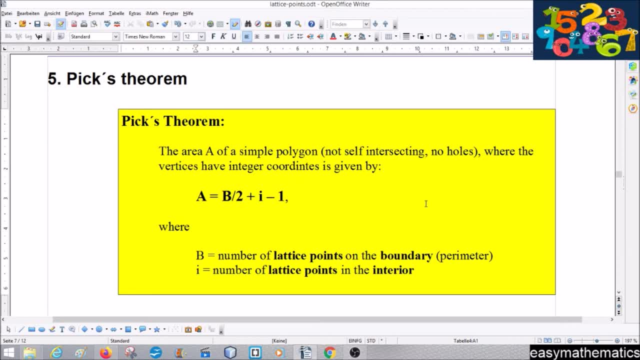 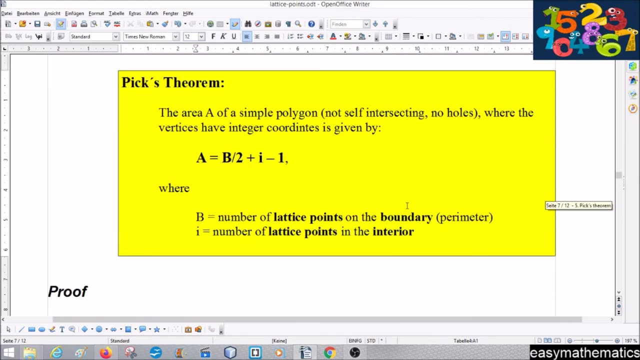 where the vertices have integer coordinates is given by the following expression: b over two plus i minus one, where b is the number of lattice points on the boundary or on the perimeter and i is the number of lattice points in the interior. Okay, 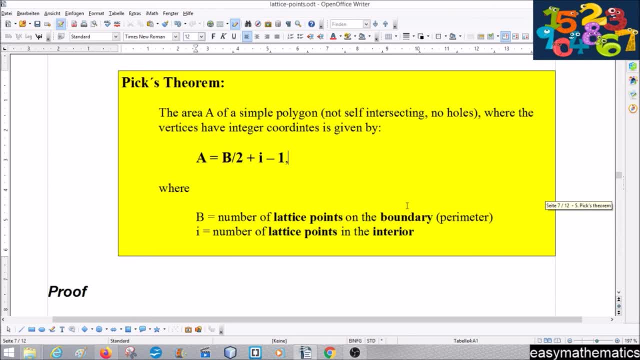 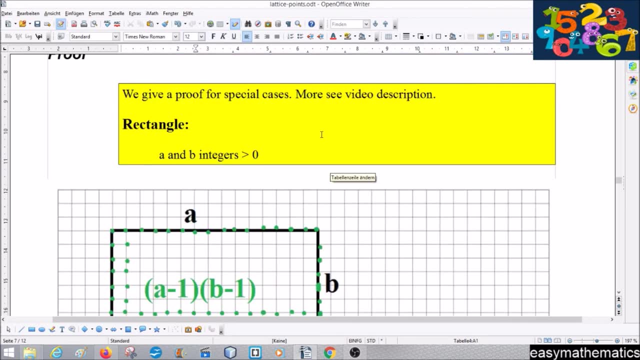 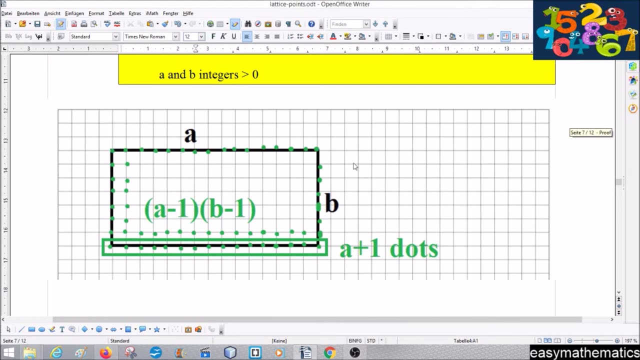 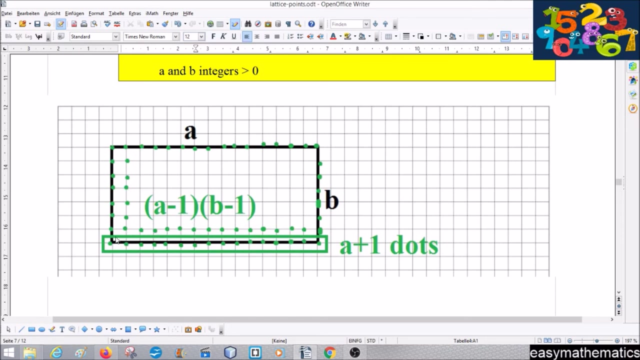 And, like I said, we will prove this for our special case And for more details, see the video description. So, if we have a rectangle, a and b are positive integers. If we have a rectangle, we count the dots here, And if the side lengths of the rectangle are a and b, 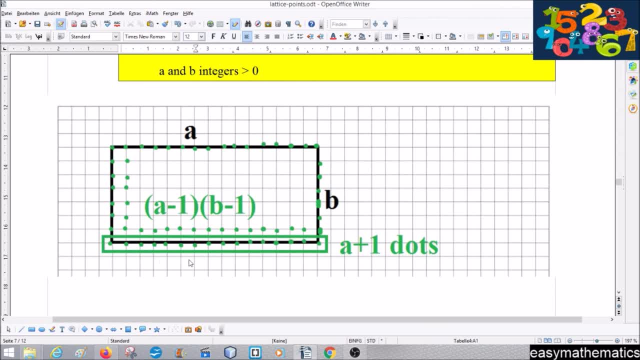 we have, for example, on the bottom line, a plus one dots. So if we leave one corner we have here a dots, then with the same argument, b dots, then a dots again and b dots again on the boundary. So we have two a plus two b dots on the boundary. 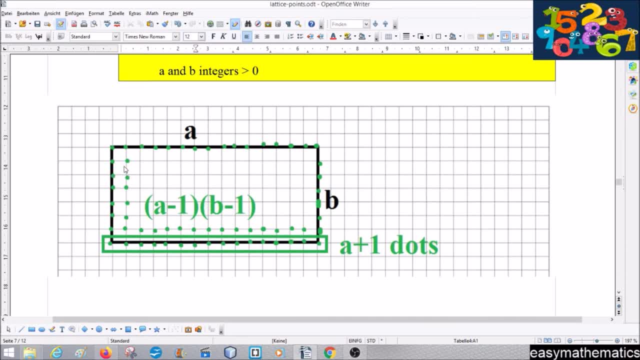 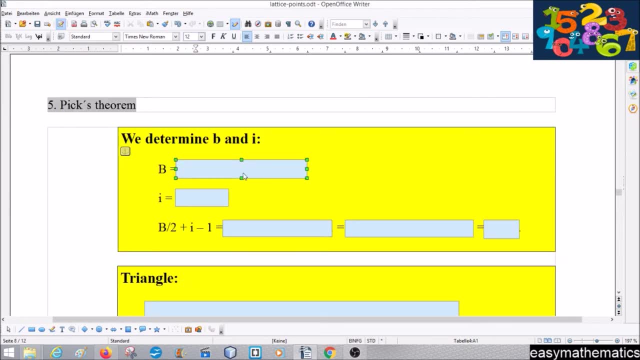 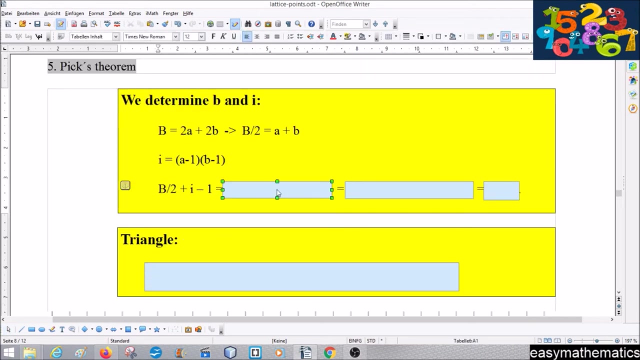 And in the interior we have a minus one times b minus one dots. Okay, Yeah, so capital B is two a plus two b, So b over two is a plus b, And the interior is a minus one times b minus one. 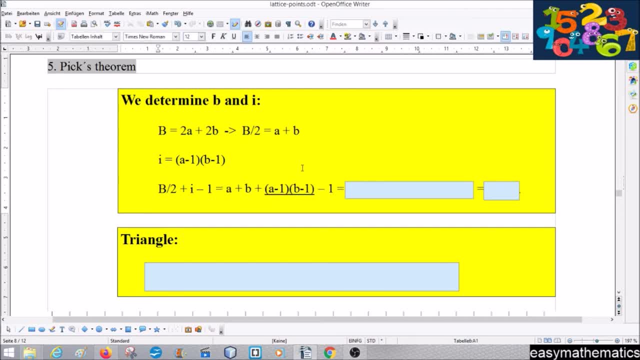 So we plug that in. We have a plus b plus a minus one, times b minus one minus one. We simplify And we see that a plus b minus a minus b cancel out. plus one minus one cancel out and we are left with a times b. 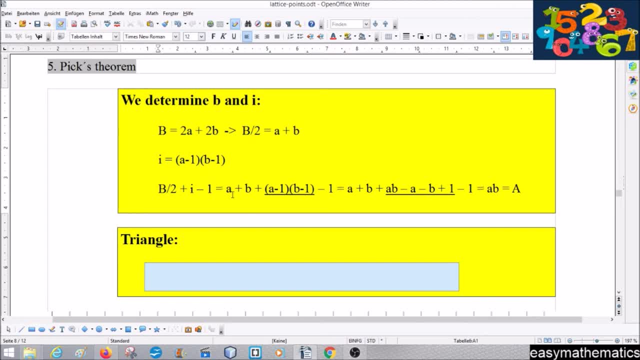 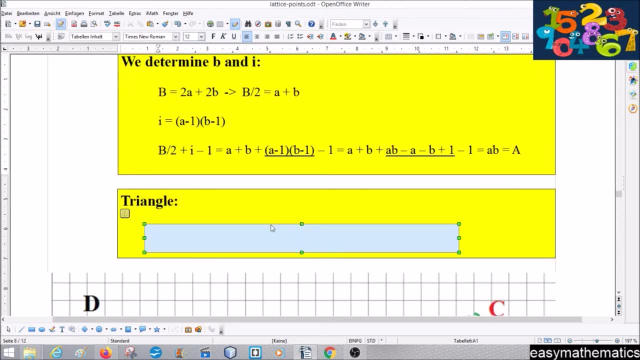 And this is the area of the rectangle. So the so Pick's theorem holds for rectangles, Okay, And for a triangle, yeah. what can we do? We cut the rectangle along a diagonal and we have to count carefully, Okay. 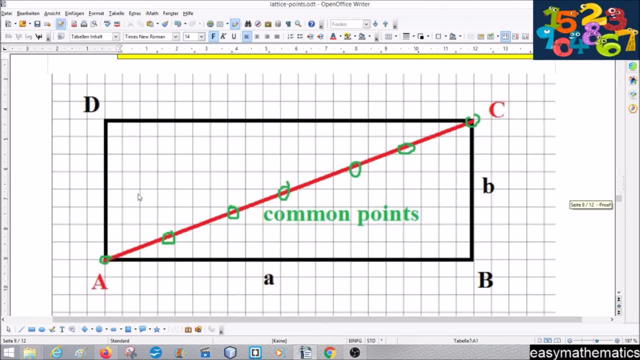 So what do I mean by that? So we know already the amount of lattice points in and on the boundary of a rectangle, And this is equal to the area of the rectangle. So if we halve them and we count the dots for each triangle 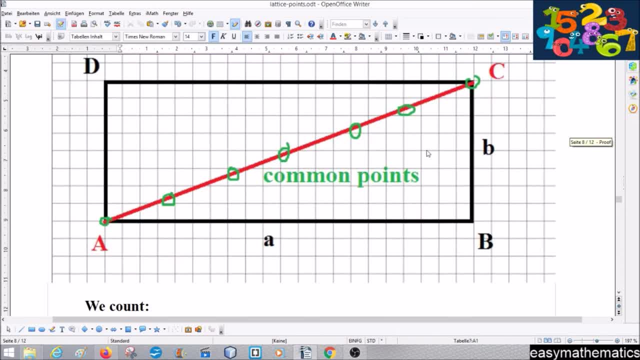 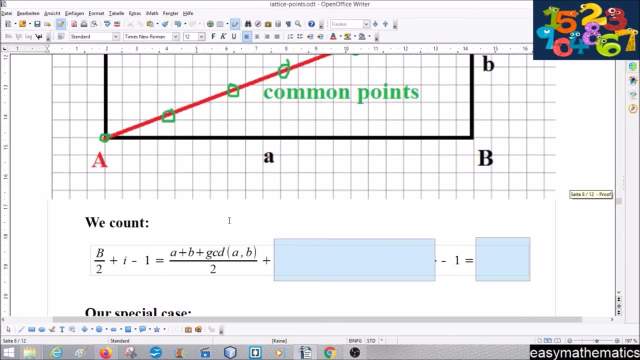 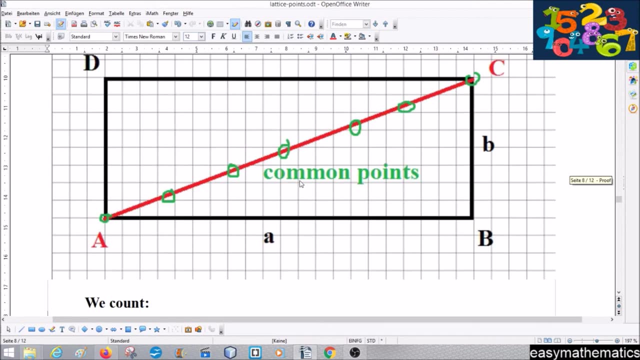 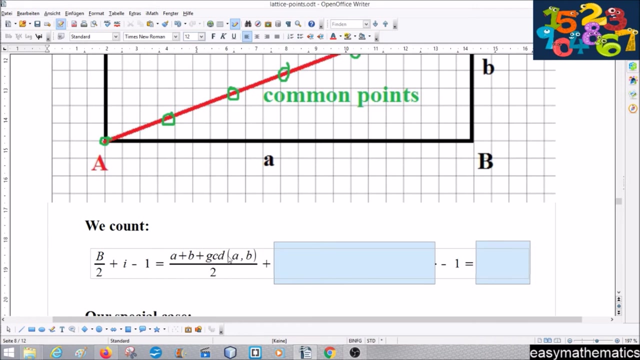 on the diagonal. we count twice. Okay. So we have on the boundary a plus b and the red line by lemma one between a and c. they are gcd minus one points on this line segment. Okay, And so therefore the sum on the boundary is: 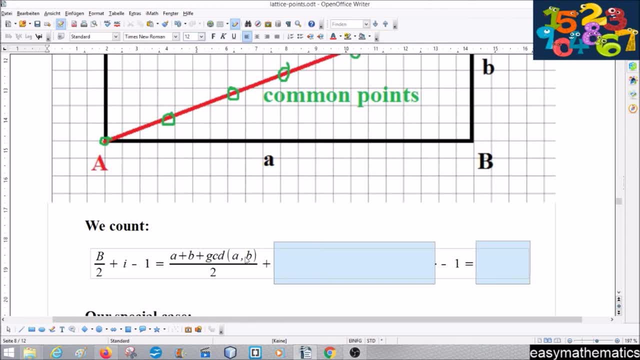 a plus b plus gcd of ab. Please make sure you got this. Then in the interior: yeah, we have a minus one times b minus one for the whole rectangle. Then we count this, the diagonal we have already counted. So we subtract gcd ab minus one. 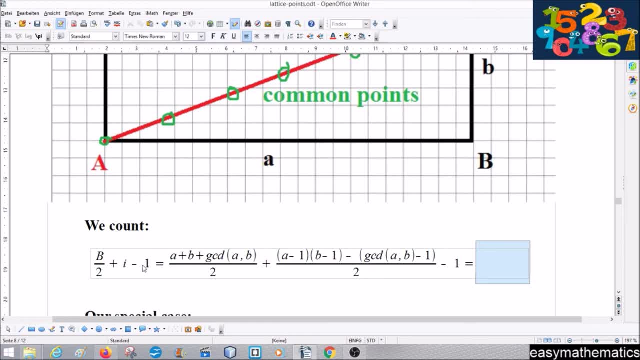 and we halve it, Okay. And then, by by pick's theorem, we subtract minus one And what we get is: if you simplify this carefully, you will see that this is indeed the area of the triangle ab over two, All right. 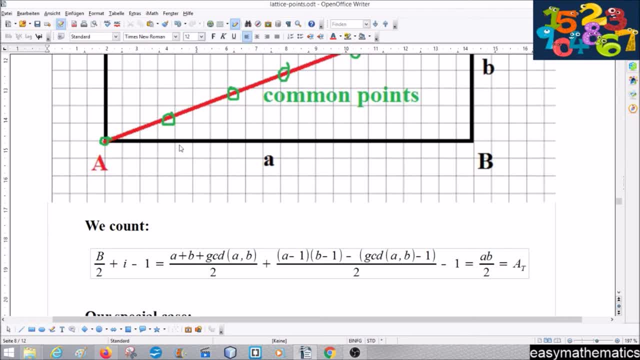 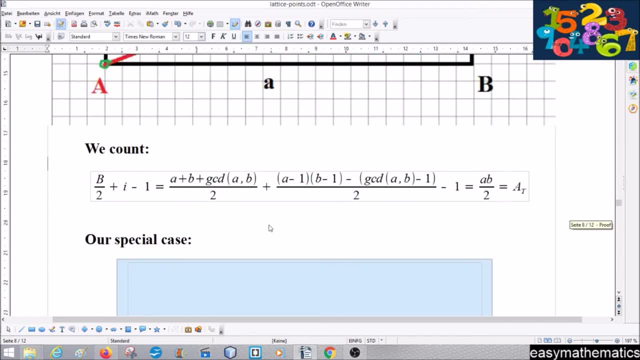 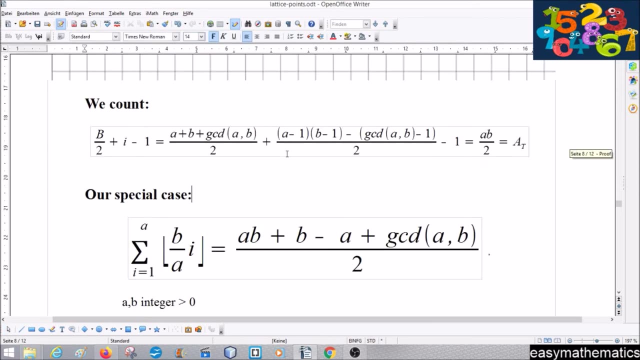 So for right triangles where the two legs are parallel to the coordinate system, pick's theorem holds All right. And now our special case is when we remember the formula above is a times b plus b minus a plus gcd, ab over two. 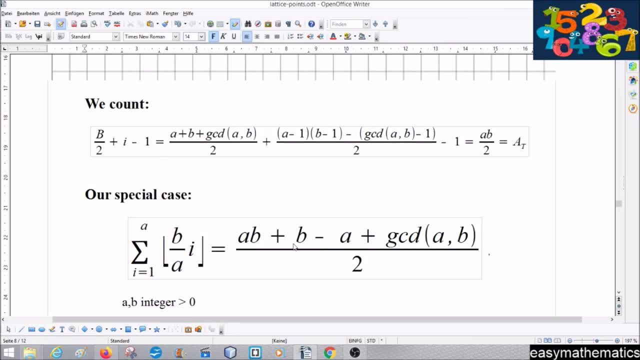 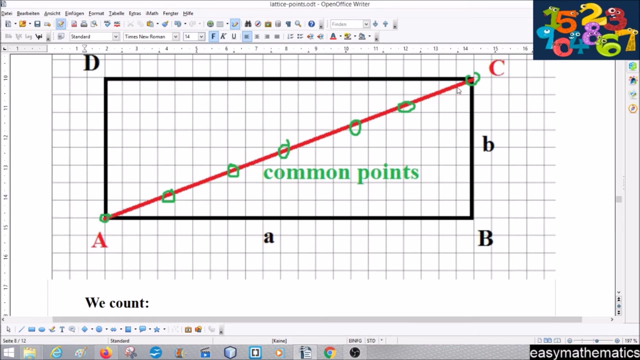 And how we can get our special case from this. We see they are quite related. They have the same, yeah, structure. But how we can find this sum? What we do is we consider this diagonal, so this red line. we consider this as a function. 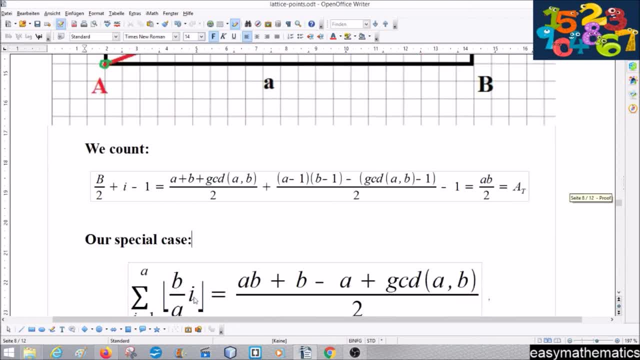 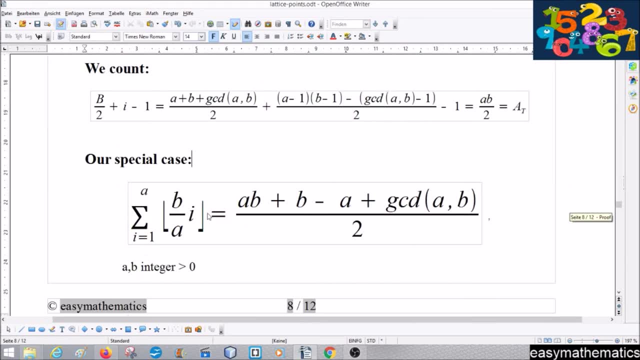 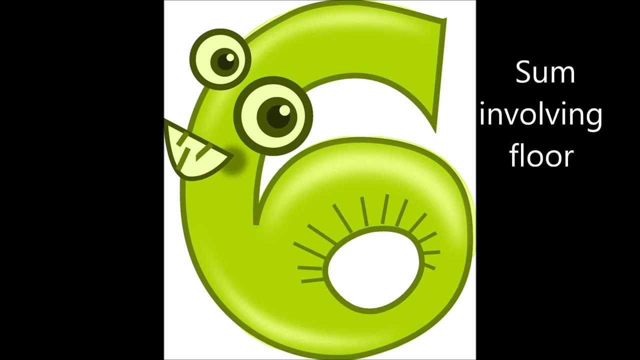 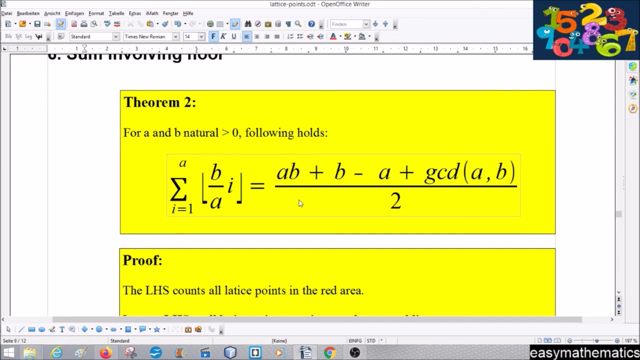 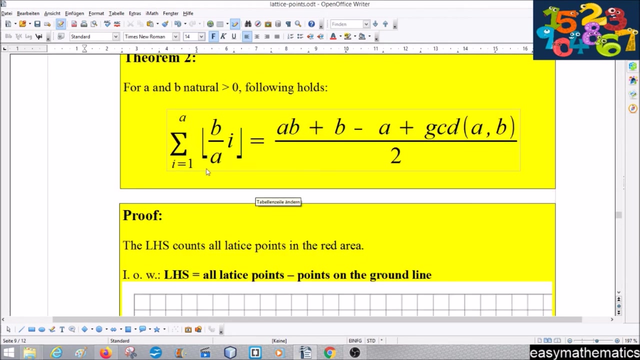 And the floor of that gives us the lattice points above the line. Okay, So think about that. So now we are ready to prove this statement here. Yeah, And again. so this sum here, the left hand side, it counts all lattice points. 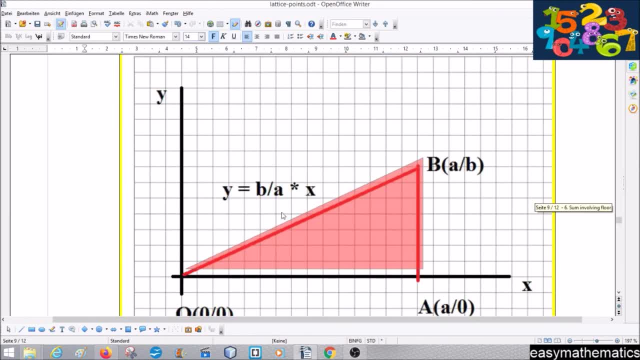 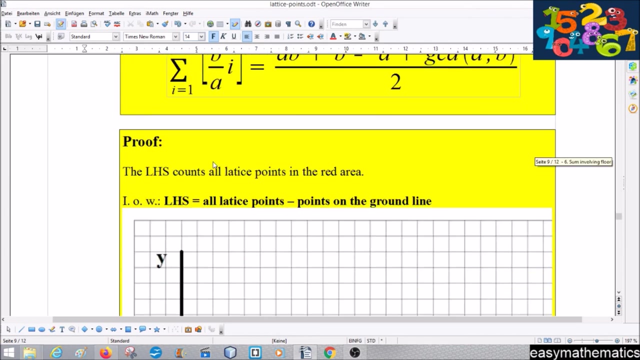 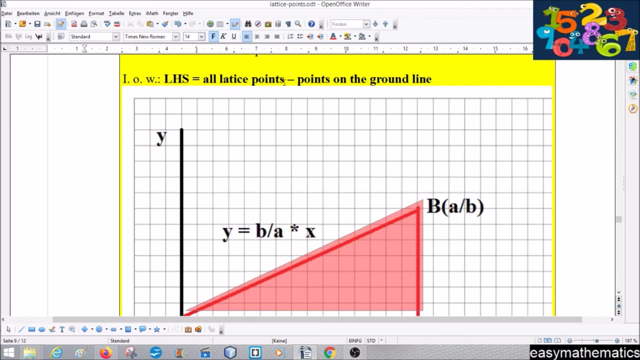 in the red area And I show this. Yeah, Please make sure it counts: all lattice points, excluded the lattice points on the on the bottom line. Okay, Yeah, Think of it, You will get this idea. Yeah, So all lattice points minus points on the ground line. 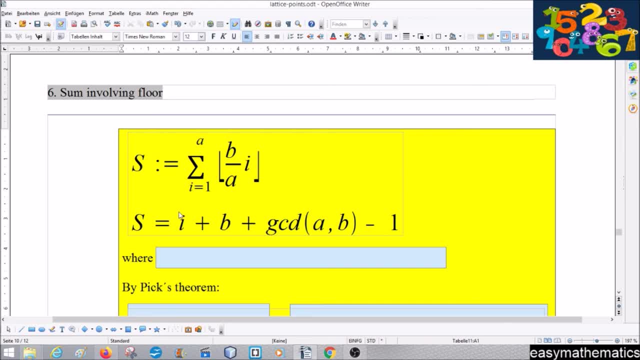 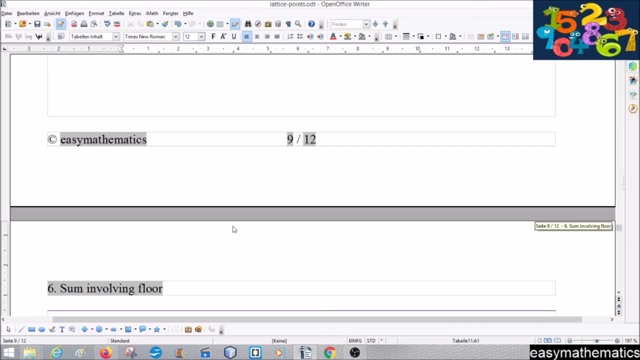 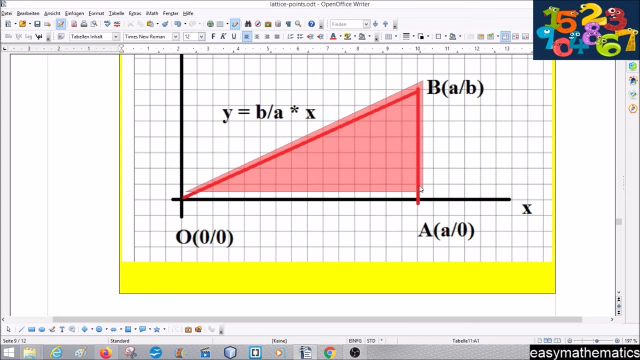 And we know already. Yeah, So the sum is the interior plus B. This is this part. Okay, So the interior plus the points on this red line, This is exactly B And the points on this red line, This is GCD minus one. 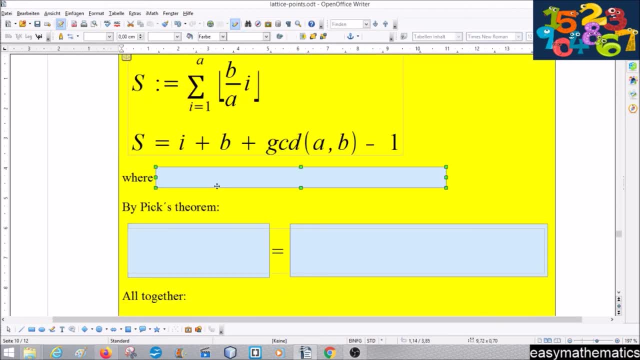 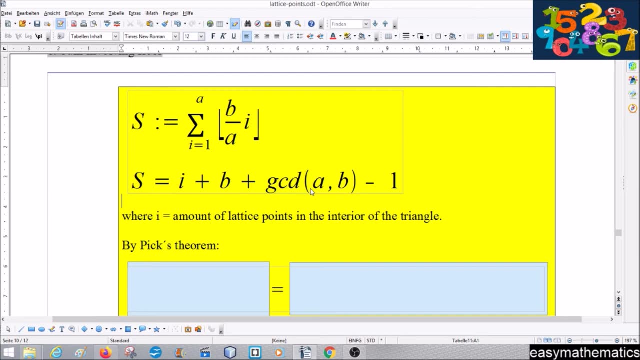 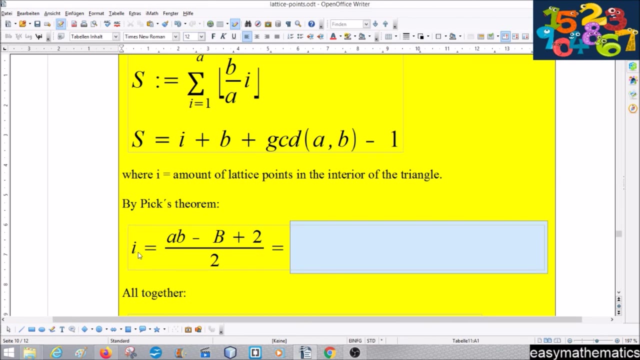 Okay, Yeah, Well, and I is the amount of the interior of the triangle. Okay, So please make sure that this is correct. And then, by Pick's theory, the interior is- we have seen that- above an AB minus the boundary. 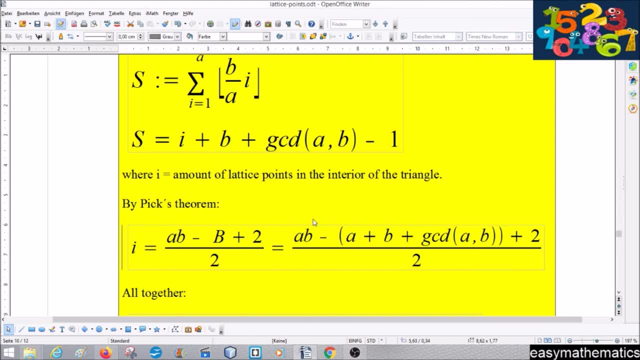 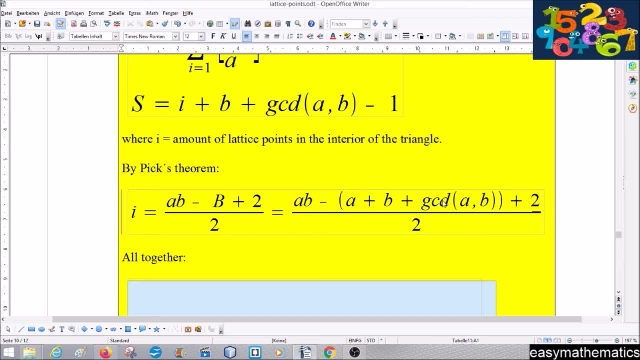 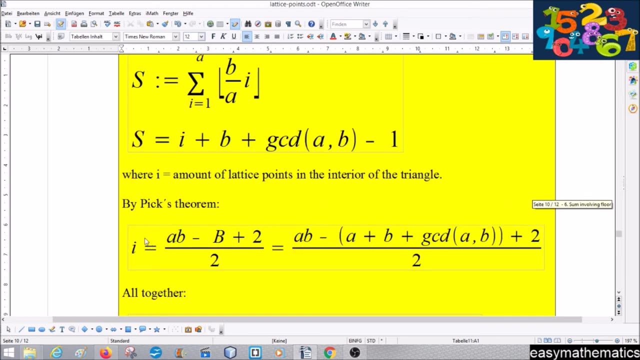 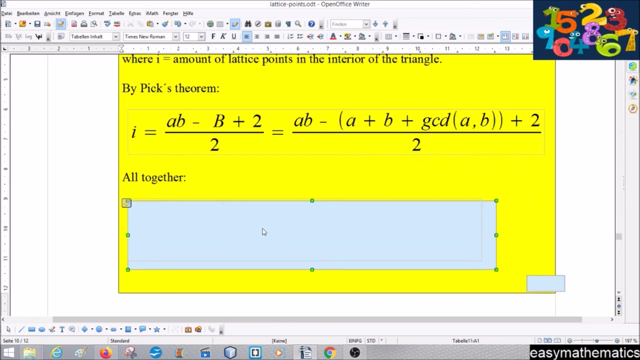 plus two over two And if we simplify that, if we plug in all values, we get this expression And all together. you see, if we plug in this interior, for here, for capital S, we get what we want. The floor sum is: 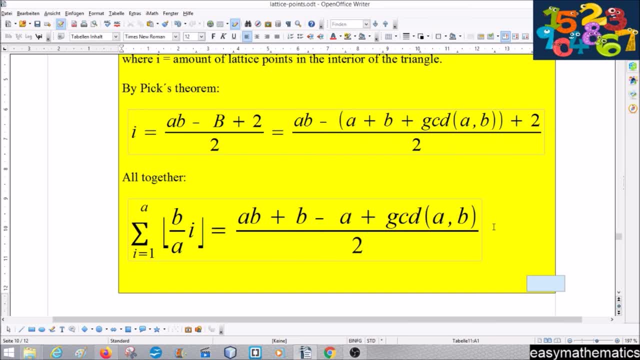 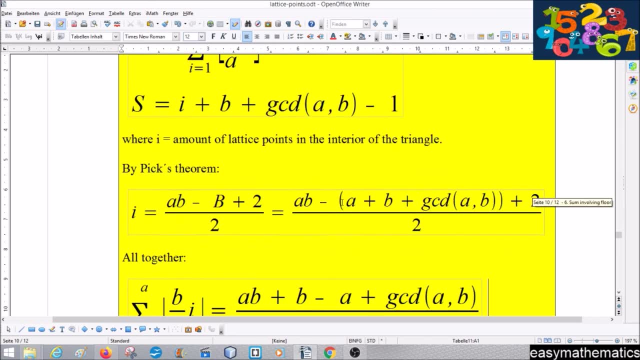 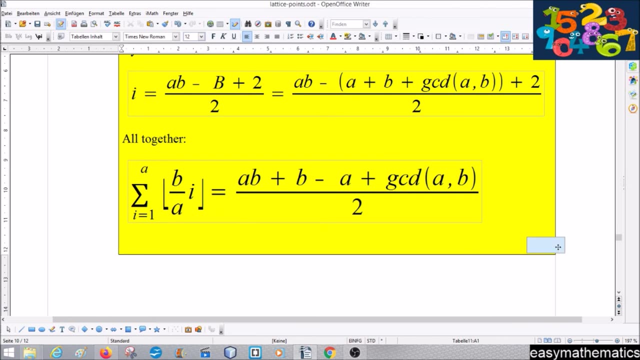 A times B plus B minus A plus GCD AB over two. Okay, So please pause the video and make sure you get all the steps. Okay, I leave small details for you. This is a very nice result in my opinion, And this finishes our proof. 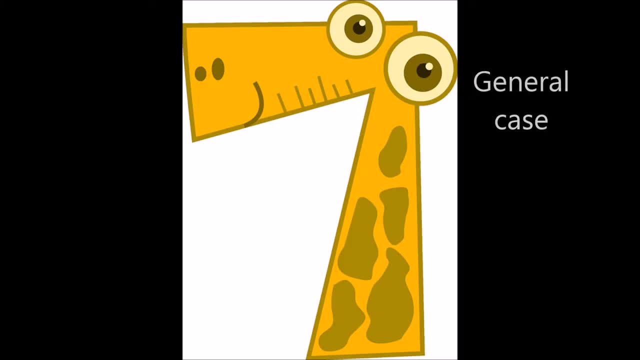 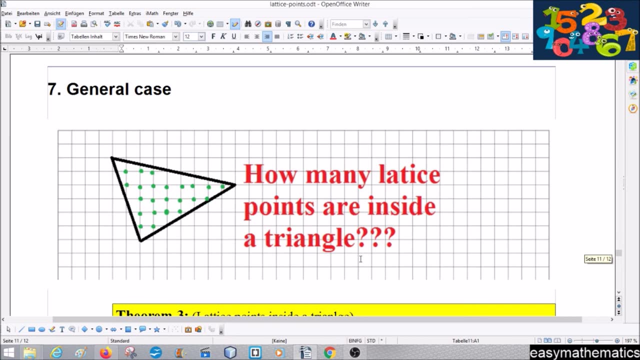 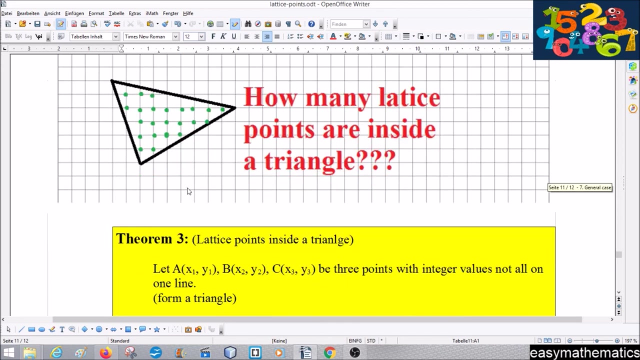 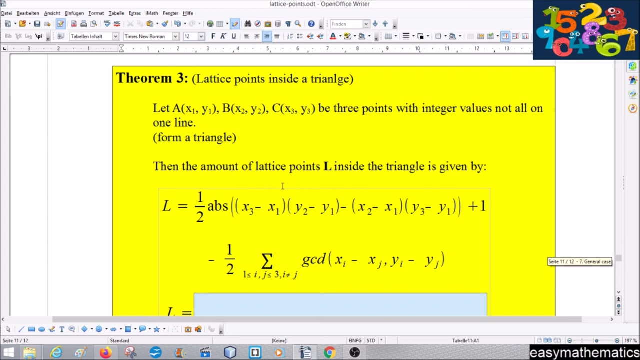 Perfect. Okay, the general case is, if we have a triangle, yeah, where the sides are not parallel to the coordinate system, and how we can, how we can count this And yeah, like I said before, this is the result. 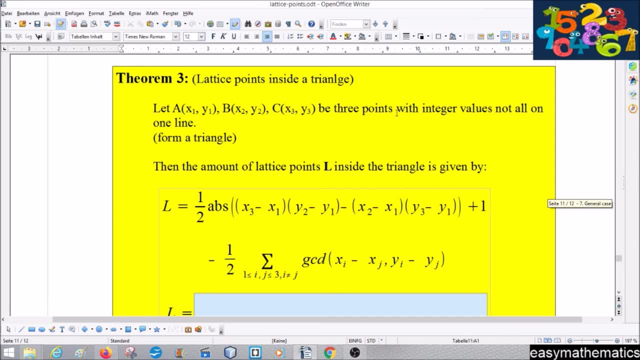 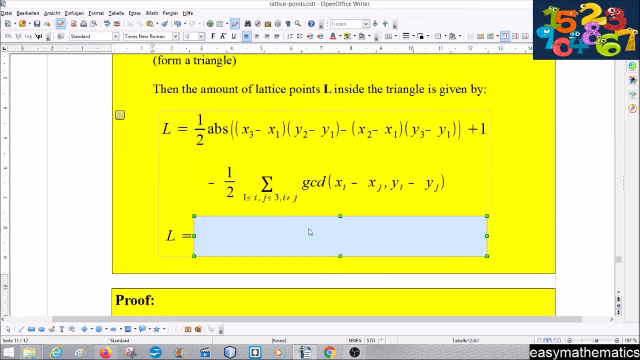 so the first result: Yeah, let A, B, C be three points with integer values, not all on one line, So in other words from a triangle. then the amount of lattice points is given by this expression, Or the first one. 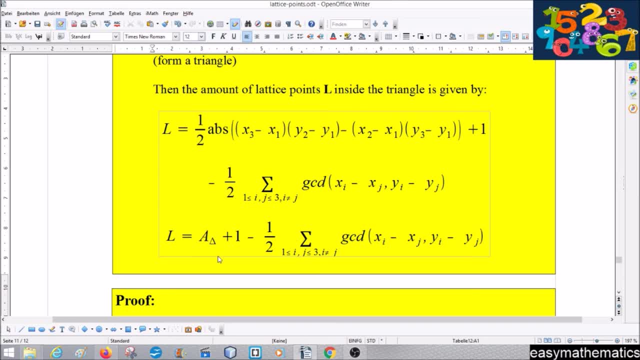 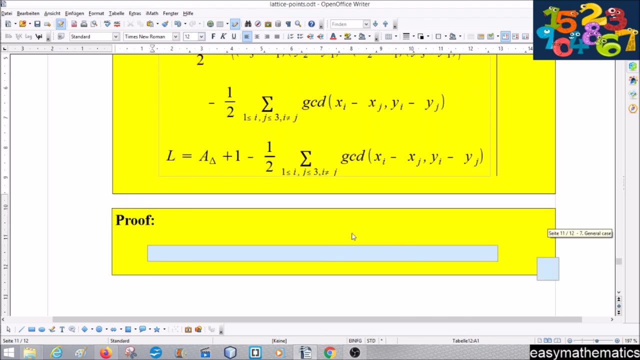 like I said, is the area of the triangle, to make it a little bit more compact. Okay, So lattice points inside the triangle is area triangle plus one, minus one half over this, minus one half times the sum, over these GCDs. Yeah, 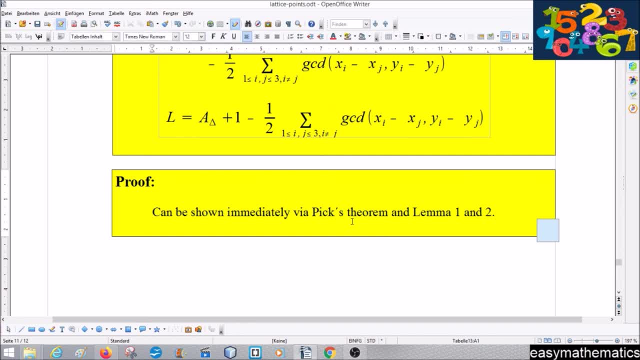 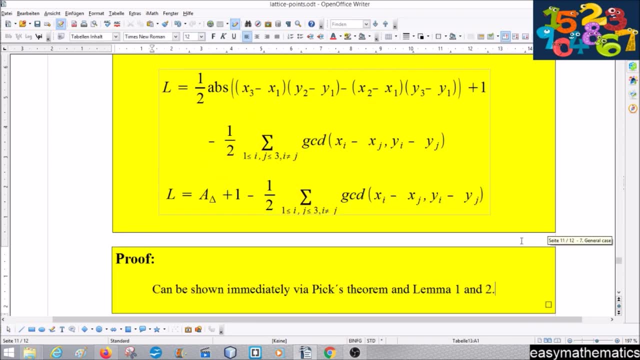 so this is the result. Now, this is the proof. It can be shown immediately via Pick's theorem and lemma one and two, And I leave this as a homework for you. Okay, we get this result immediately with Pick's theorem and lemma one and two. 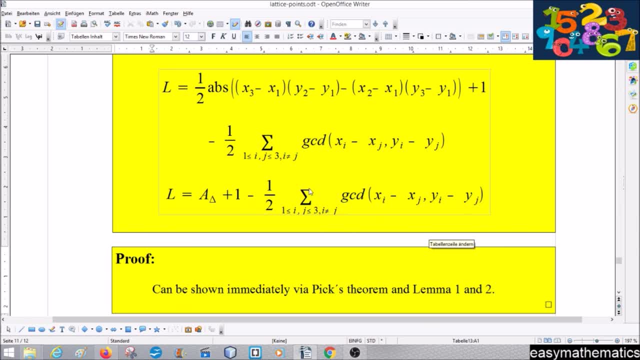 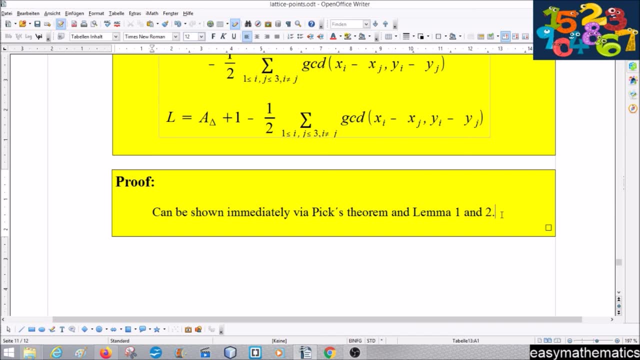 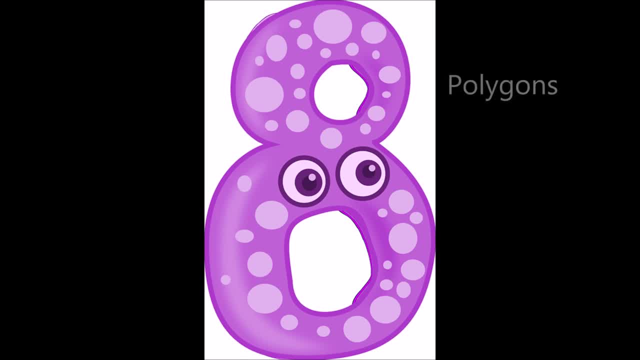 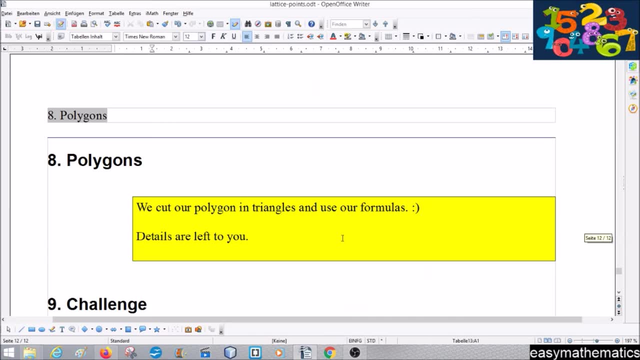 Bye, Bye, Bye, Bye, Bye, Bye. And for polygons: we cut our polygon in triangles and use our formulas. Details are also left to you. Yeah, So you know that a polygon. we can cut this polygon in smaller pieces. 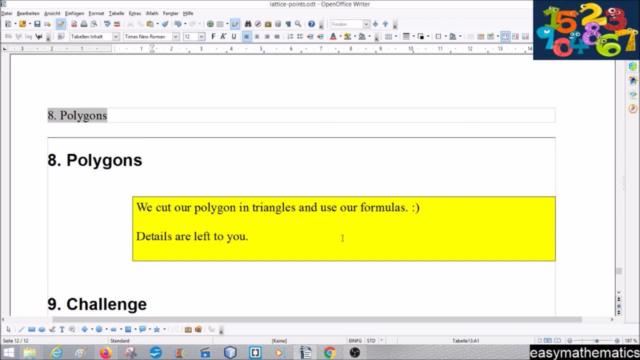 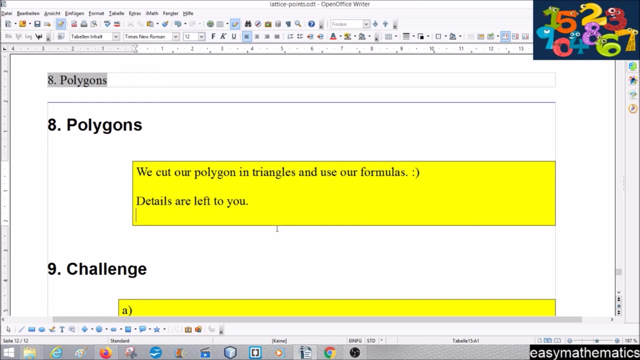 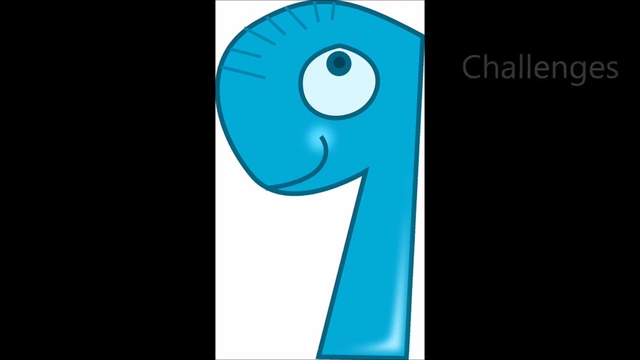 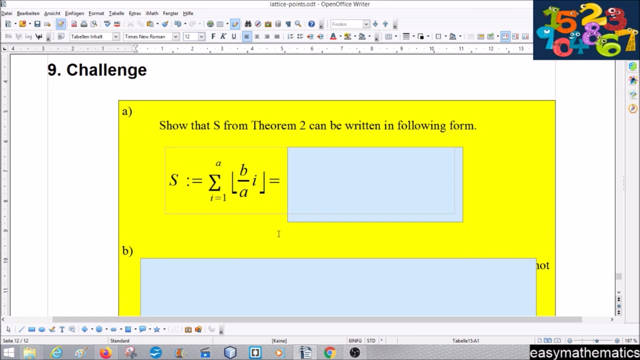 The smallest pieces are the triangles, and for triangles we have a formula and then we put them all together. you will find also very nice formulas in the internet if you look by yourself. i will not write this down here. yeah, and the last point. the challenges show that s from theorem two can be written in following form: 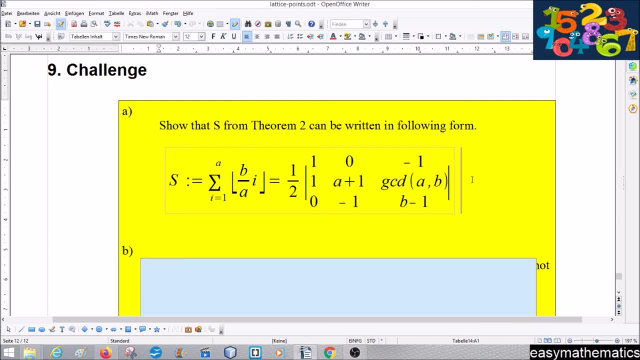 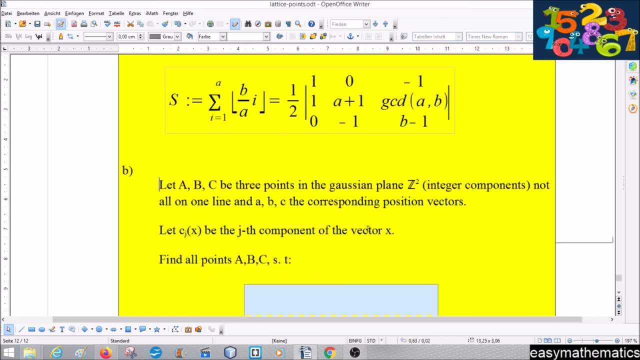 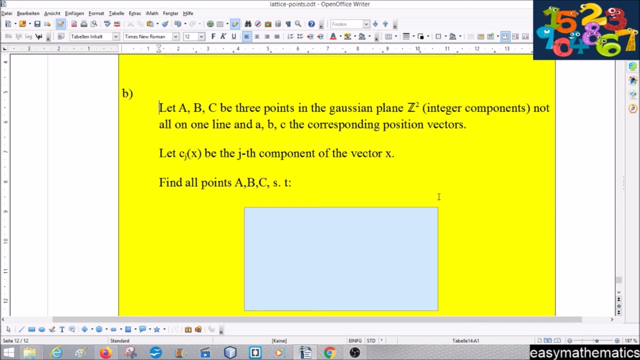 yeah, one half times this determinant. i will not read all the columns, you can read it by yourself. and b, yeah, let a, b, c be three points in the gaussian plane set squared, so an integer components, not all on one line, and small- a, b, c, the corresponding position vectors. 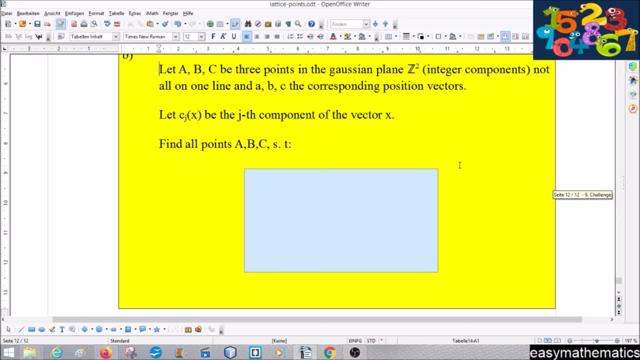 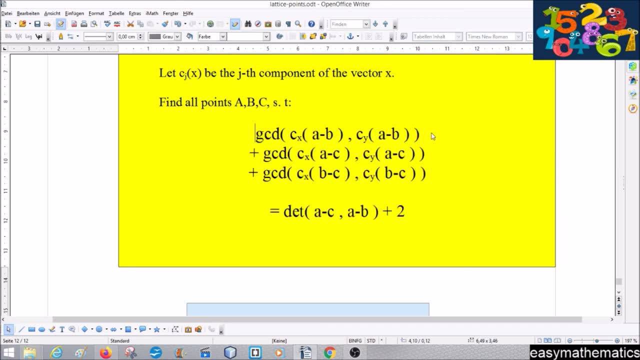 let c, j of a, c, j of x be the jth component of the vector x, find all points a, b, c, such that what g, c, d of c, x of a minus b and c, y of a minus b plus g, c, d and plus g. 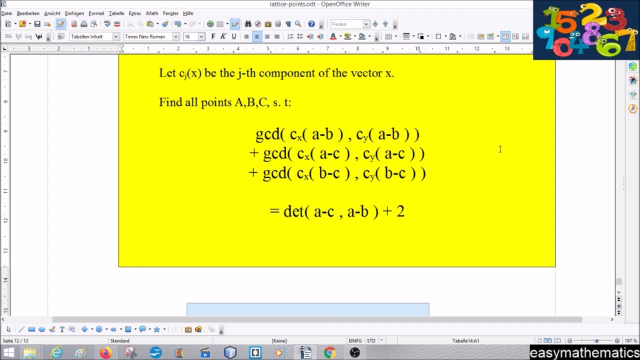 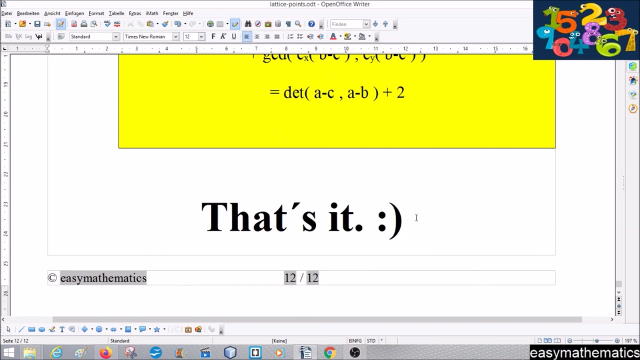 c, d, so all the three gcds of the vector components of the sides is equal to the determinant spanned by the vector a minus c and a minus b plus two. okay, i want all coordinates satisfying this equation. yeah, that's it. thanks for watching. hope you liked it and 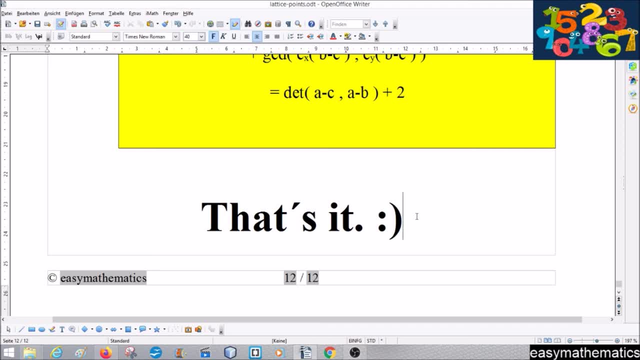 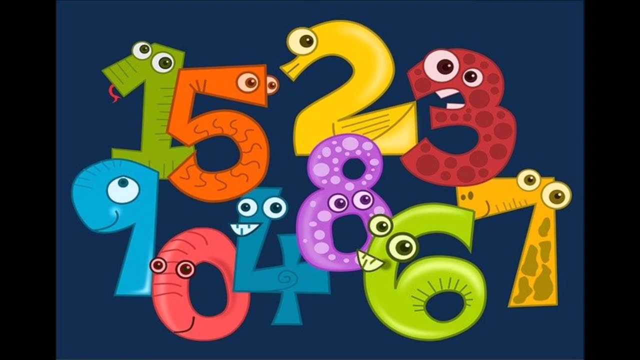 if you, if you have seen the last challenge with the gcd, this comes from one of those equations. so see you next time. enjoy, bye, bye you.